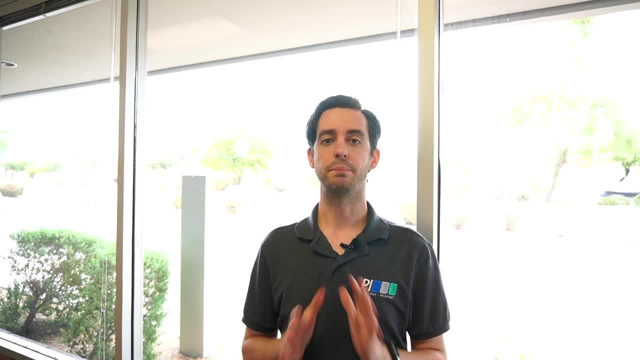 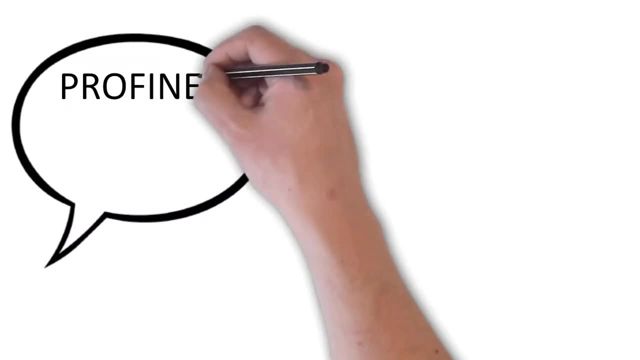 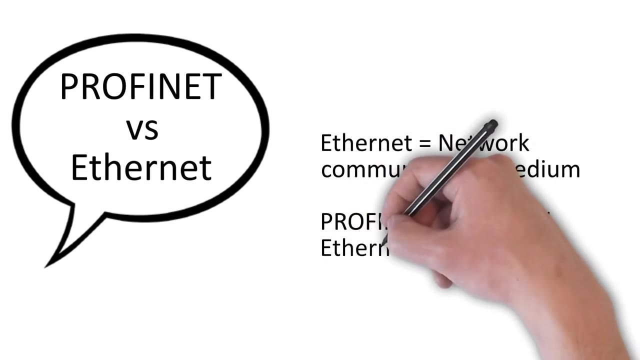 to this channel. But for now let's go to the whiteboard for a complete PROFINET versus Ethernet comparison. What is the difference between PROFINET and Ethernet? In short, Ethernet is a network communication medium and PROFINET is an industrial Ethernet. 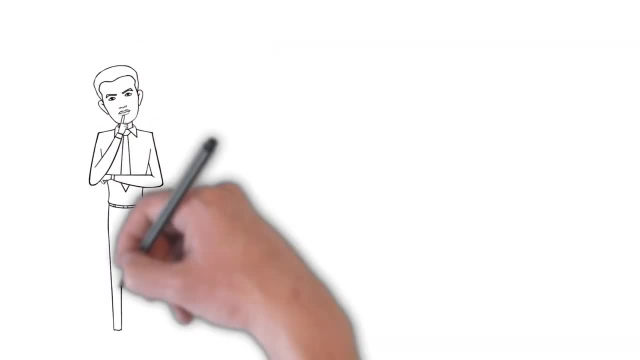 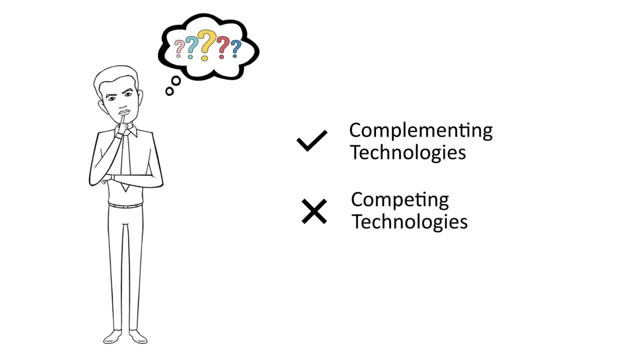 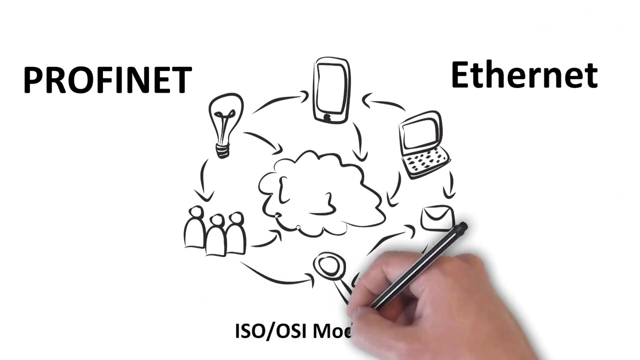 standard. However, comparing Ethernet and PROFINET is not easy because they are complementing technologies, not competing technologies. They fulfill different tasks within a communication system. We can explain this by introducing the ISO-OSI model. So what is the ISO-OSI? 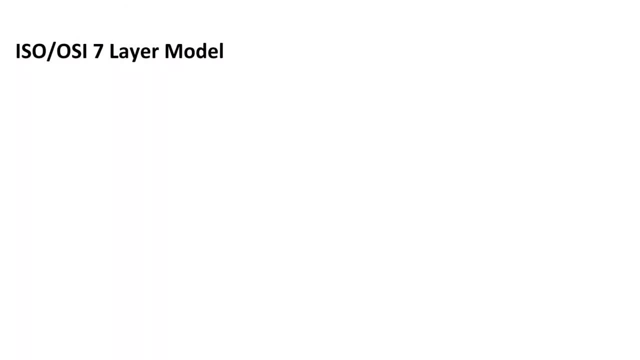 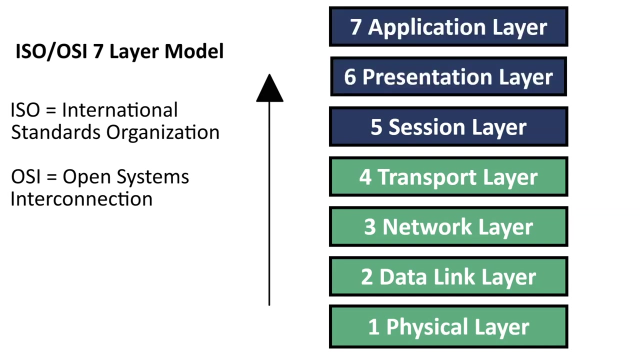 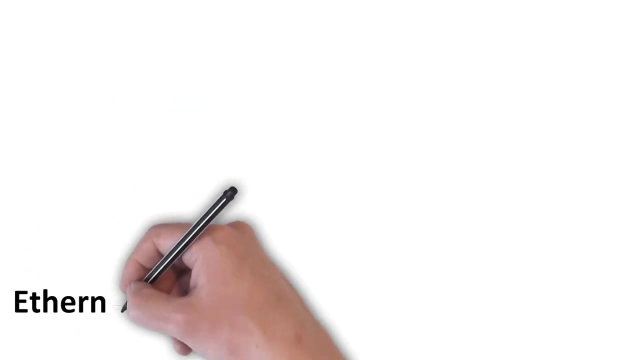 model. It is a seven-layer model that generically describes the abstraction layers of a communication system From bottom to top. the seven layers are the physical data link, network, transport, session, presentation and application. Each of these layers has a specific function. Where do Ethernet and PROFINET sit in this model? Ethernet lives. 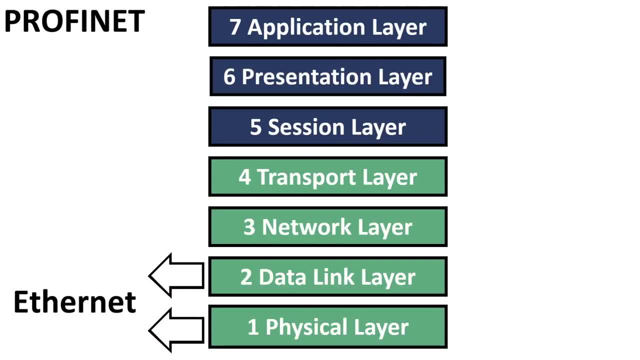 at layers one and two and PROFINET at layer seven. Layer one and layer two are all about generating electrical signals, accessing the bus and sending and receiving signals. The seven-layer model, on the other hand, is the top layer and it describes the application. 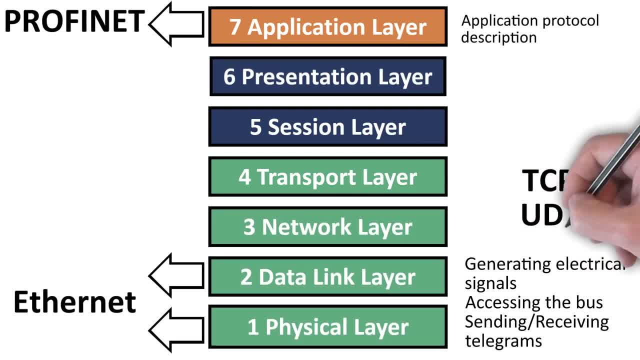 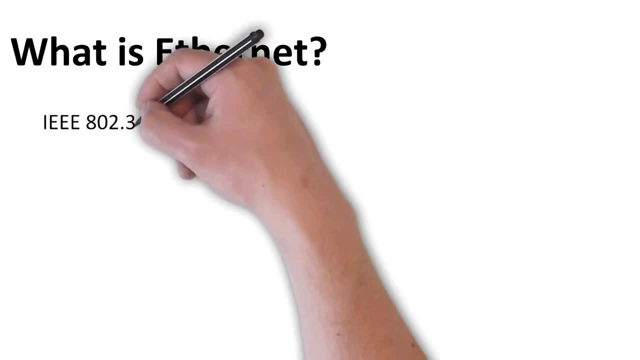 You might also be familiar with TCPIP or UDPIP. They both reside on layers three and four of the model network and transport. Now let's explain Ethernet and PROFINET separately and then put those concepts together. What is Ethernet? IEEE 802.3 specifies the standards. 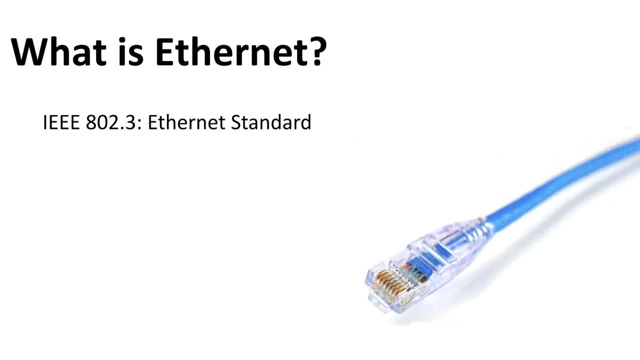 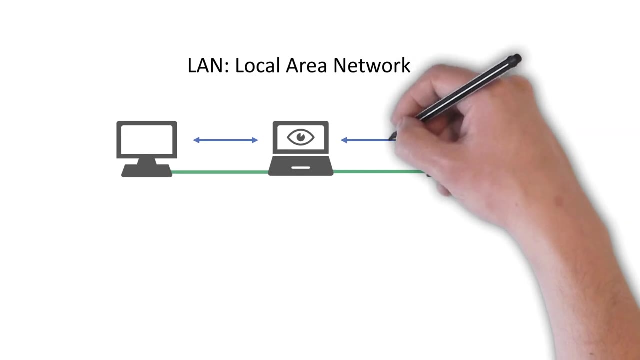 that make up Ethernet. Ethernet frames include information such as the MAC addresses of the sender and receiver, virtual LAN tagging and quality of service. Ethernet is used to connect nodes in a local area network. The physical link between nodes in an Ethernet network can be, for example, 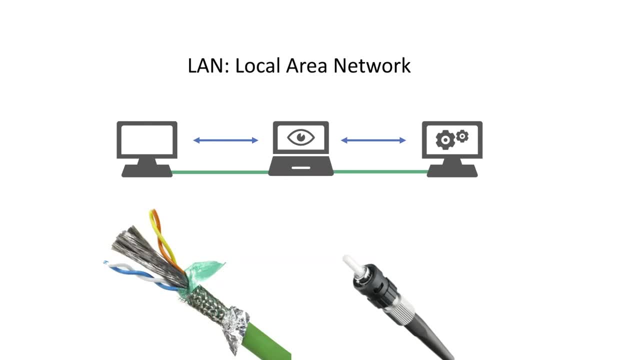 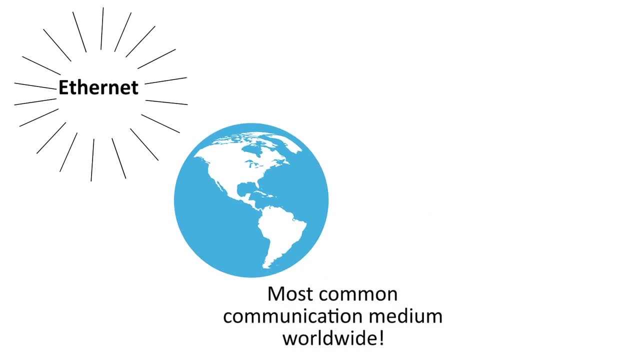 a twisted pair cable or a fiber optic cable. Nowadays, Ethernet is the most common communication medium worldwide, used in homes, enterprises and in general infrastructure, due to its speed, affordability and versatility. PROFINET is an industrial Ethernet solution. It is a communication protocol designed to 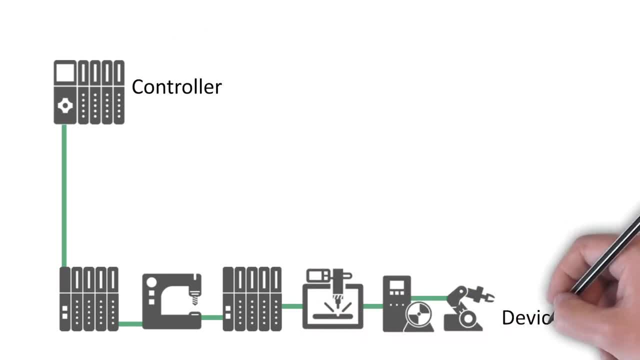 exchange data between controllers and devices in an automation setting. PROFINET defines cyclic and acyclic communication between components, including diagnostics, functional safety alarms and additional information To link all of those components. PROFINET is a highly-demanded technology. It can be. 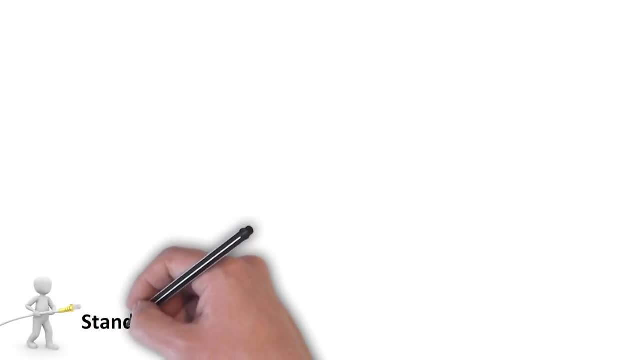 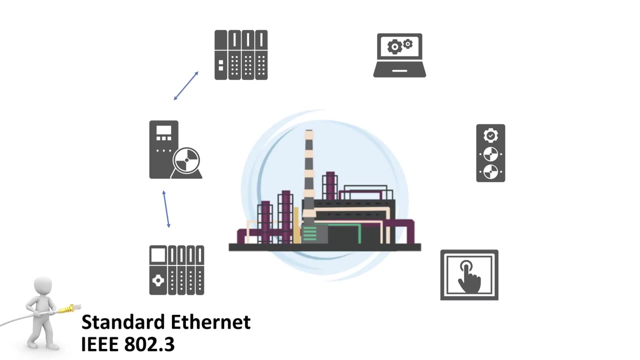 used in a number of different ways. For example, it can be used in a number of different ways. First, PROFINET employs standard Ethernet for its communication medium. If you encounter a PROFINET network, you will notice the Ethernet cables connecting PROFINET components. 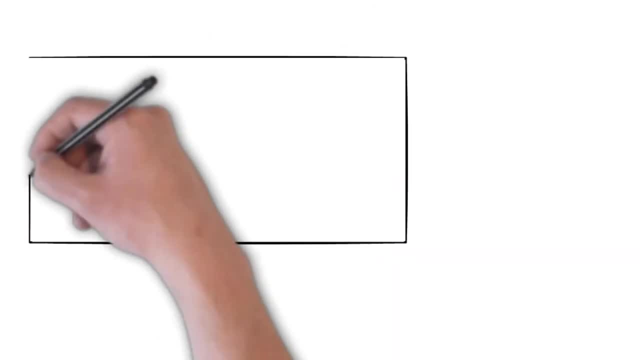 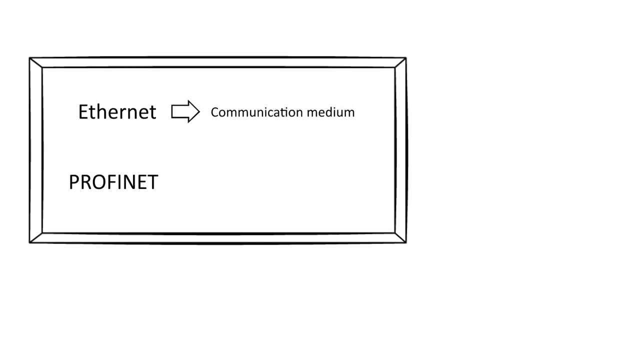 So today we learned that PROFINET and Ethernet complement each other. They are both in industrial networks: Ethernet as the communication medium and PROFINET as the protocol. Now let's answer some common questions to clear up any outstanding doubts. 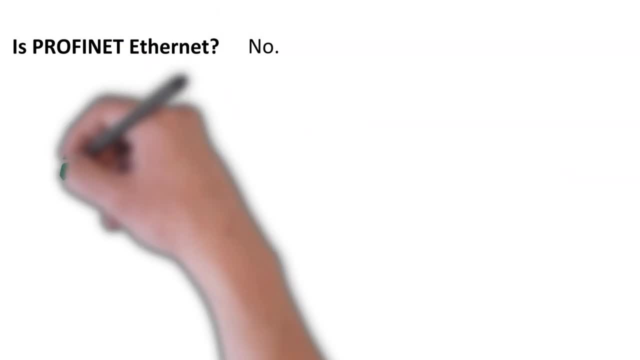 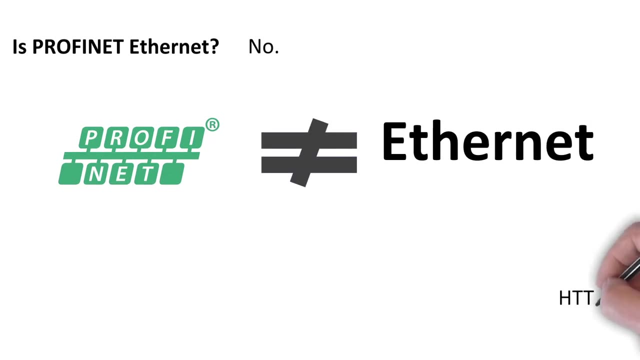 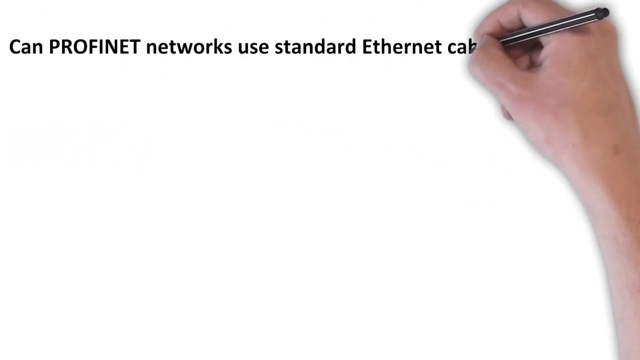 Is PROFINET Ethernet? No, PROFINET is an application that is based on Ethernet. Comparing PROFINET to Ethernet would be like comparing HTTP, OPC, UA or any other application to Ethernet. Can PROFINET networks use standard Ethernet cables? 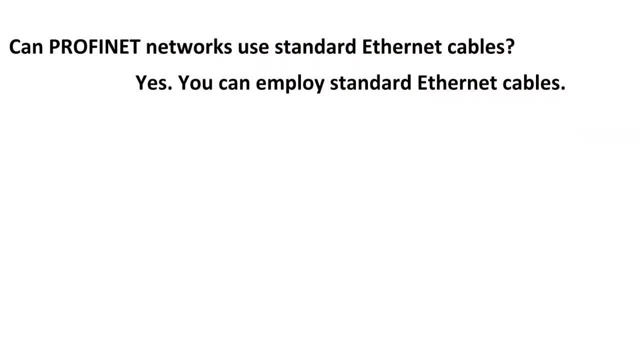 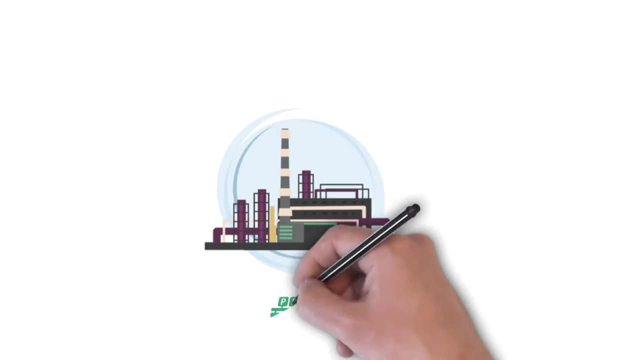 Yes, you can employ standard Ethernet cables to build a PROFINET network. However, the Ethernet cables that you might encounter in a home or office environment might not be the best choice. Those cables can be weak and might lack shielding The factory floor where PROFINET is most commonly. 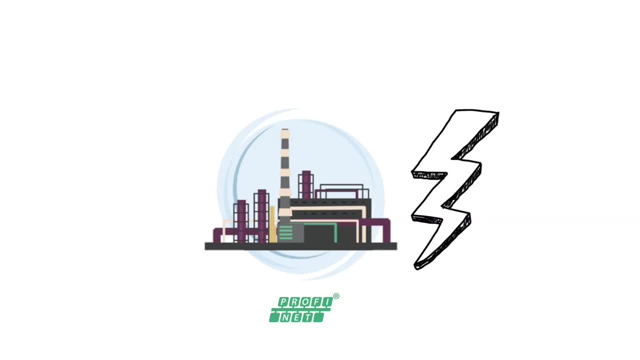 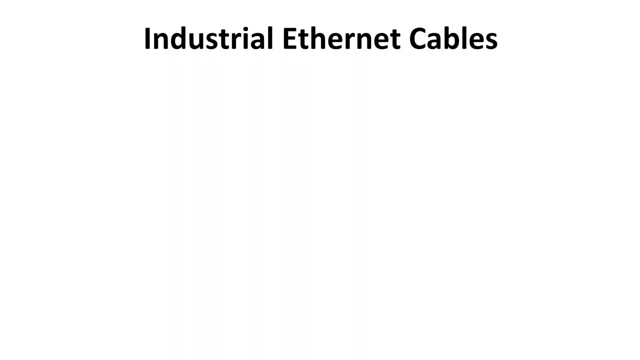 used can be a rough environment with challenging conditions such as extreme temperatures, humidity, vibrations and electromagnetic interference. These reasons, even though you can employ standard Ethernet cables, it is recommended to use industrial Ethernet cables On the wire. they are the same thing, Yet industrial Ethernet is characterized by ruggedized hardware shielding. 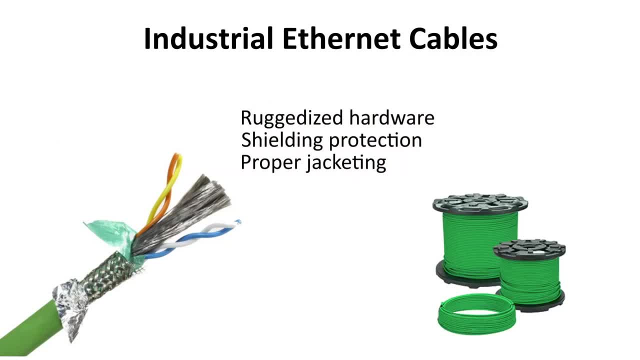 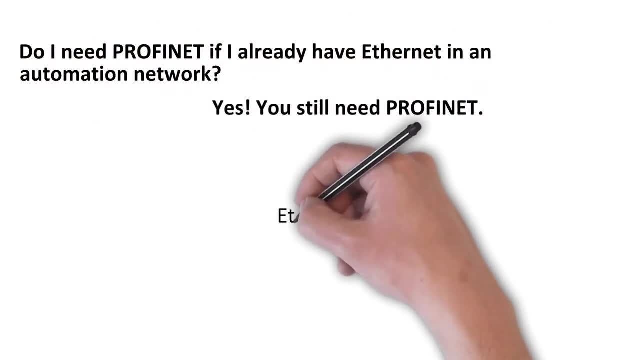 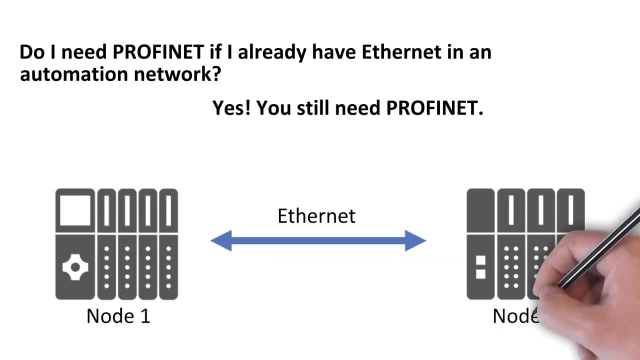 protection and proper jacketing. Do I need PROFINET if I already have Ethernet in an automation network? Yes, you still need PROFINET. You create a connection if you link two nodes in a network with an Ethernet cable. but there is so much more than just linking those two components.